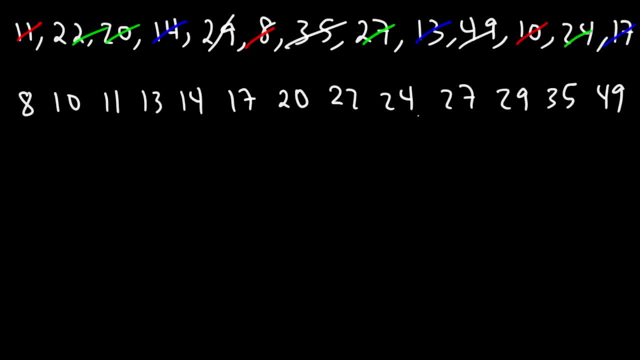 So at this point we have a total of 13 numbers. So we can see that we have a total of 13 numbers in our list. Now the first thing is to break the data into two equal parts. So let's calculate Q2,, which is the median of the entire data set. 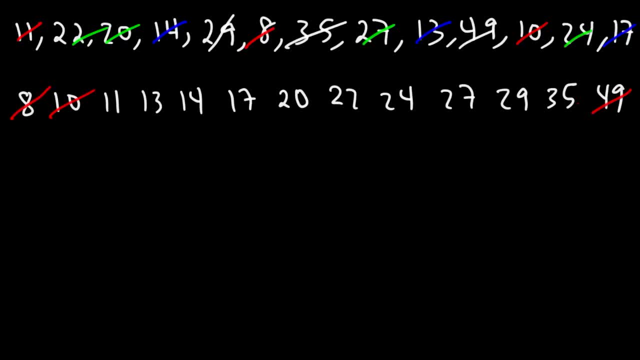 So if we eliminate the first two numbers on both sides and then if we keep doing that until we get the middle number, this will give us the median, which is 20.. Now what I'm going to do is I'm going to draw a line and then put 20 on top. 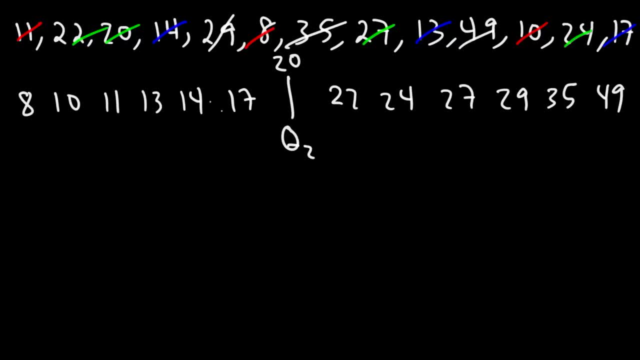 So this is the second quartile. So now I have two equal parts of data. I have six numbers on the left side and six numbers on the right side. Now I need to find the median of the lower half of the data. So if I eliminate the first two and the last two, I mean the next two. I have two numbers in the middle. 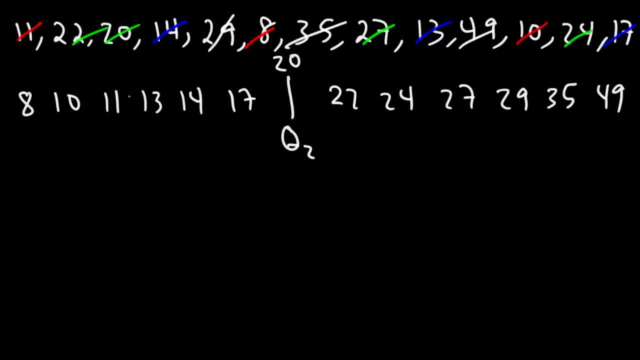 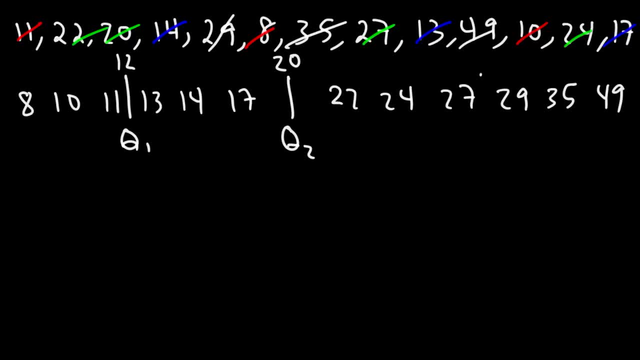 So this is Q1, the first quartile. Now the median will be between these two numbers, That is the median of the upper half of the data. So the average of 27 and 29 is 28.. So that's Q3, the third quartile. 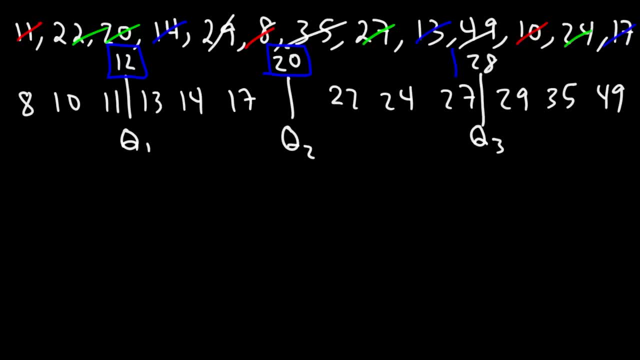 So we have Q1,, Q2, and Q3.. Now the next thing we're going to do is we're going to do the median of the upper half of the data. Now, the next thing we're going to do is we're going to do the median of the upper half of the data. 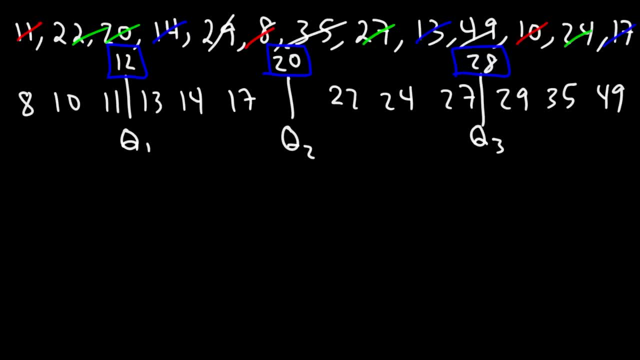 So the first thing we need to do is identify the minimum value and the maximum value. The minimum value is the lowest value in the data set, which is 8.. And the maximum value is the highest value in the data set, which is 49.. 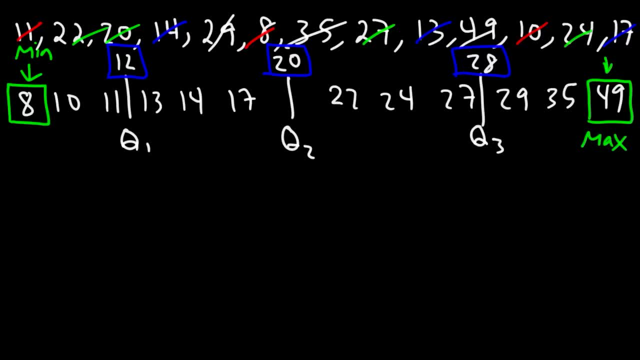 Now we need to check to make sure that these two values are not outliers, Because if they're outliers, they're not going to be part of the box and whisker plot. They will exist outside of that. Now what we need to do is we need to determine a range of numbers in which the outliers can't be. 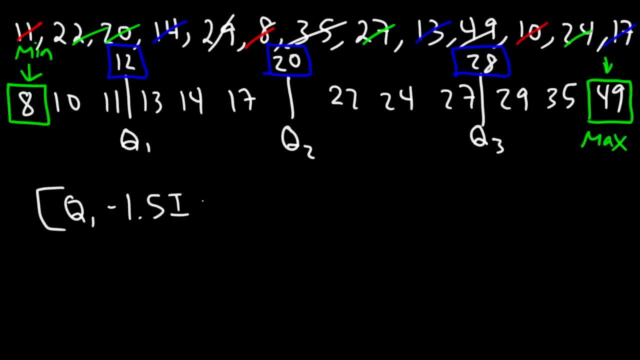 So it's going to be Q1 minus 1.5 times the IQR value to Q3 plus 1.5 times the IQR value. So any number that is outside of this range that is part of the data set is an outlier. 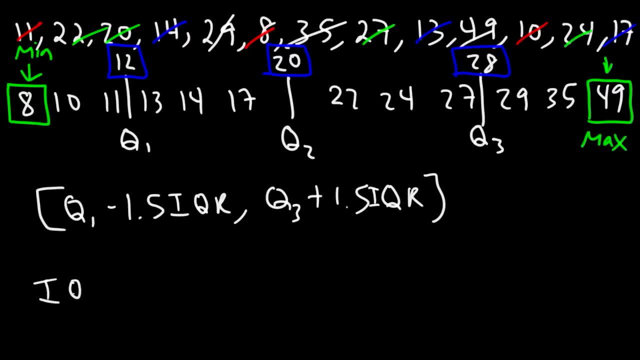 Now the IQR value. the interquartile range is basically the difference between Q3 and Q1.. So Q3 is 28,, Q1 is 12.. So the interquartile range is 16.. So, using this interval, it's going to be Q1,, which is 12, minus 1.5 times 16.. 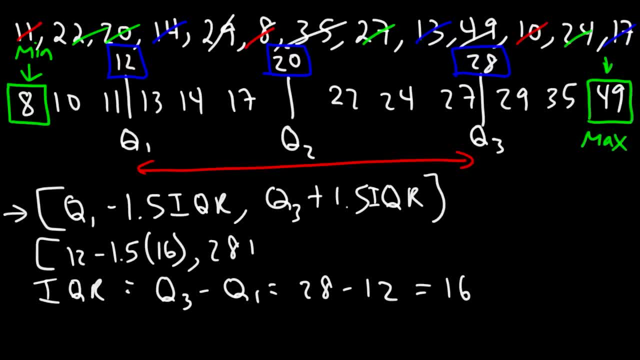 And then Q3 is 28.. Plus 1.5 times 16.. Now let's get a calculator and plug these numbers in. So 12 minus 1.5 times 16,, that's going to be negative 12.. And then 28 plus 1.5 times 16,, that's 52.. 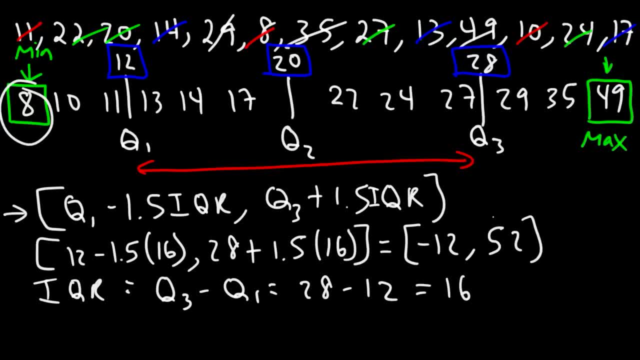 So negative- I mean not negative 8, but 8 is in this range, So 8 is not an outlier. It is the minimum of the data set. 49 is also between negative 12 and 52. So 49 is not an outlier. 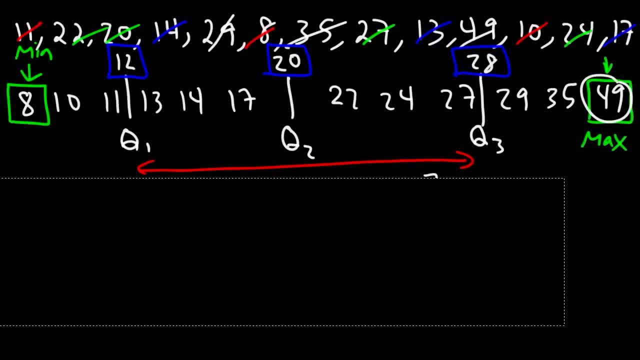 So now that we know we don't have any outliers at this point, we can draw the box plot or the box and whisker plot. Let's begin by creating a number line. The lowest value is 8 and the highest is 49.. 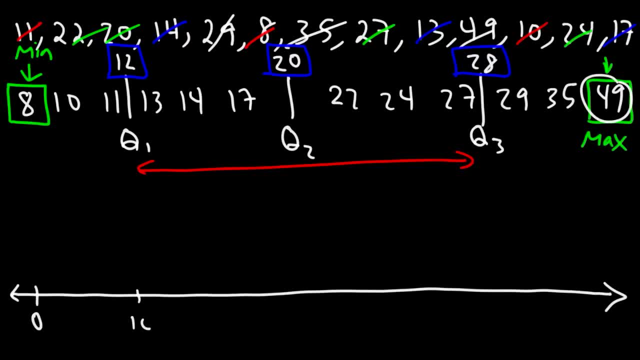 So let's start from 0.. And let's go by 10s until we get up to 50.. So first let's plot Q1.. Q1 is 12,, which is approximately right there, And then Q3 is 28,, which is just under 30. 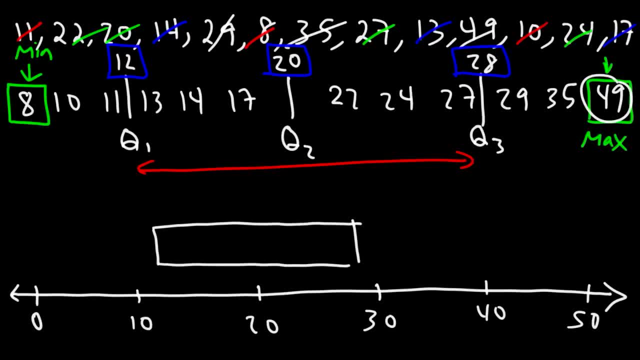 And then draw a rectangle. Now, Q2 is 20, so we're going to put a line here. So, as you can see, this is Q1.. Q2 and Q3.. Now our next step is to plot the minimum, which is around 8.. 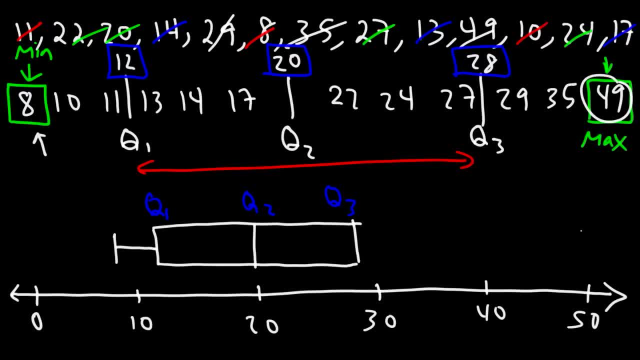 So there it is, And then the maximum is at 49. So we're going to put a line just below 50. And so that is the box and whisker plot that corresponds to the data set that we see here. So that's how you can draw it. 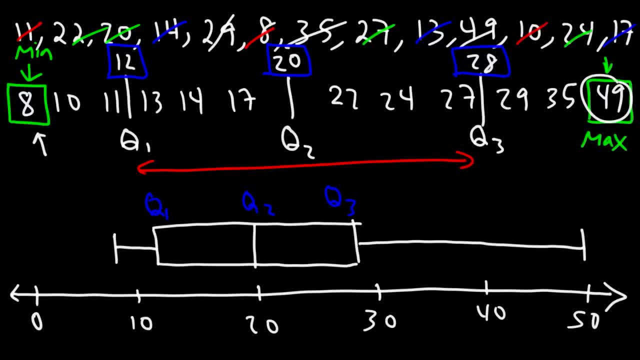 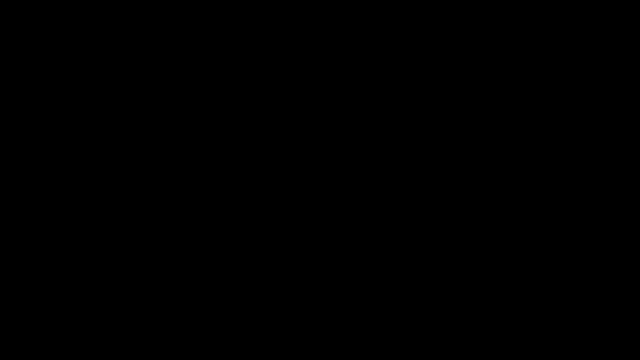 But now what about if we had an outlier? How would that impact the box and whisker plot? So let's consider an example in which that's the case. So first let's write out a list of numbers. Let's say we have the numbers 18,, 34,, 76,, 29,, 15,, 41,, 46,, 25,, 54,, 38,, 20,, 32,, 43, and then 24.. 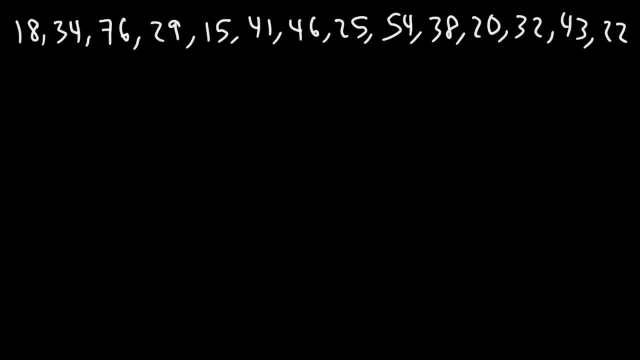 So if you think you know what to do, feel free to pause the video and try it. So let's begin by putting the numbers in ascending order. So we have 15,, 18,, 20.. And so here are those numbers. 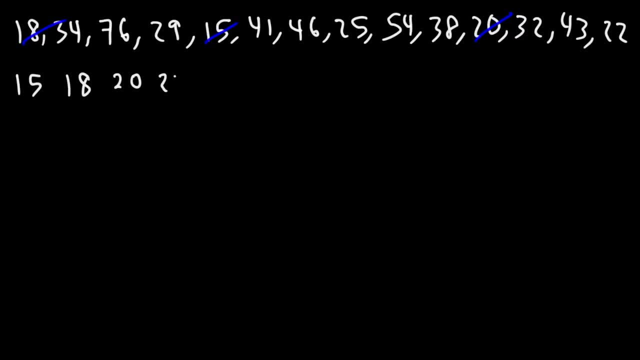 And then, after 20,, it's 22,, and then 25, and then 29.. After 29,, it's 32,, 34,, 38, and 41. And then, after that, it's going to be 43,, 46,, 54,, and then the last one is 76.. 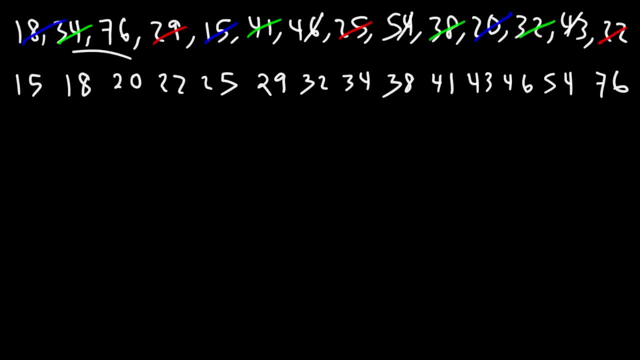 So we have a total of- let's see this is 3,, 6,, 9,, 12,, 14 numbers. So we want to split it into two equal parts. Let's put a line between the 7th and the 8th number. 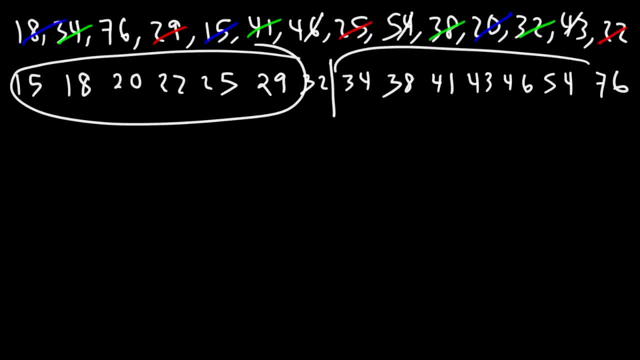 So we got 7 numbers on the left side, 7 numbers on the right side. So the median is going to be the average of those two numbers. The average of 32 and 34 is 33.. So this is the second quartile. 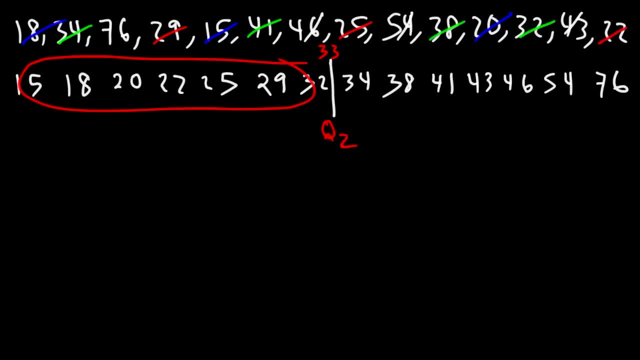 Now we need to determine the median of these 7 numbers, which is going to be the middle number, 22.. But let's replace 22 with a line So we can split the left side into two equal parts of three numbers. 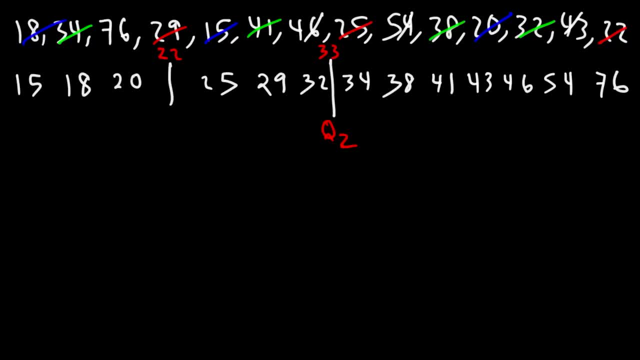 But I'm going to put 22 on top So you can see that it represents Q1, the median of the left side of the data. Now, 43 is the middle number of these 7 numbers. So let's do the same thing. 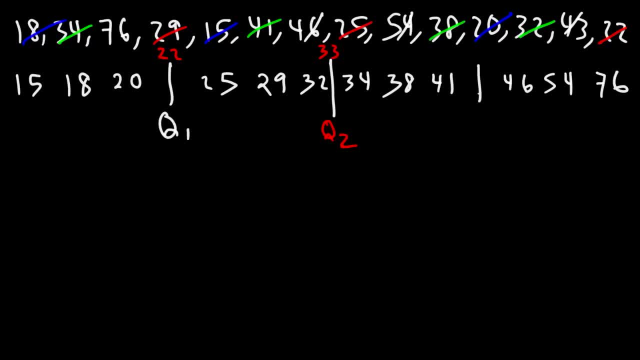 Let's replace 43 with a line, And so this is going to be the third quartile And we'll put 43 on top. So keep in mind the quartiles. they divide their data into four equal parts, So we have: 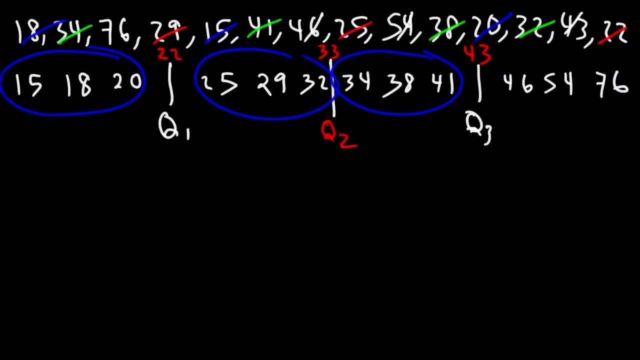 So we have four equal parts of three numbers. Now I'm going to put a comma between 46 and 54.. So it doesn't look like 4,654.. Our next step is to calculate the interquartile range. So it's Q3 minus Q1.. 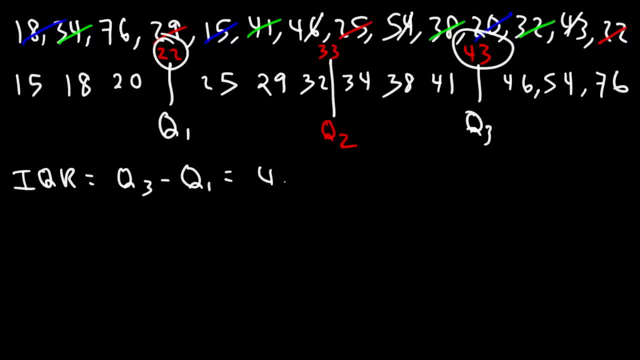 So it's the difference between those two values. So it's 43.. Minus 22,, which is 21.. So that's our IQR value And, excuse me, our next step is to see if we have any outliers. 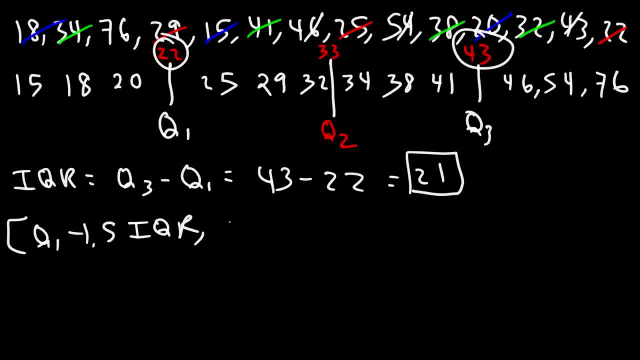 So first let's calculate the range in which no outliers should exist. So Q1 is 22. And IQR is 22. And IQR is 21.. Q3 is 43.. 22 minus 1.5 times 21.. 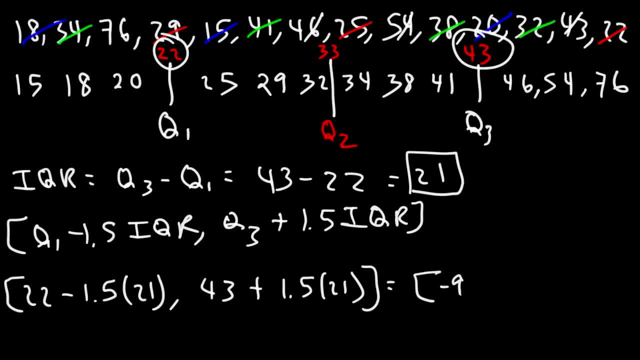 That is equal to negative 9.5.. And then 43 plus 1.5 times 21 is 74.5.. Now our score is: Our score is: Our score is: Are there any numbers in our list of numbers that is not in this range?